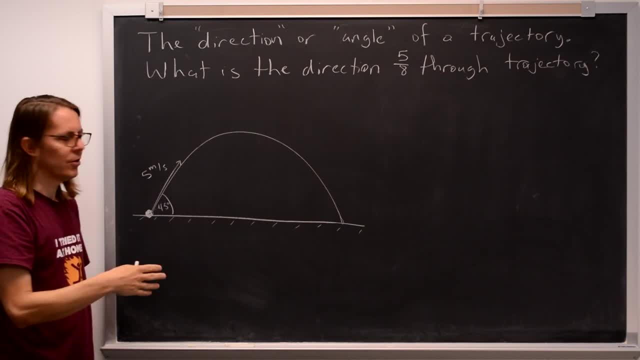 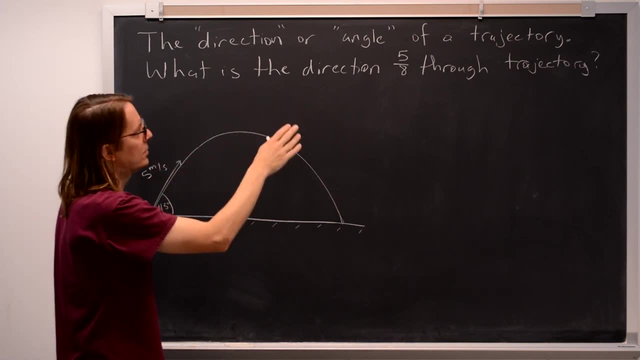 ground, making it an even trajectory, an even projectile, so that we can use our standard range and hang time formulas. But the question we're trying to answer is: what is the direction of the path 5? eighths through the entire trajectory. So that's just to make it a little. 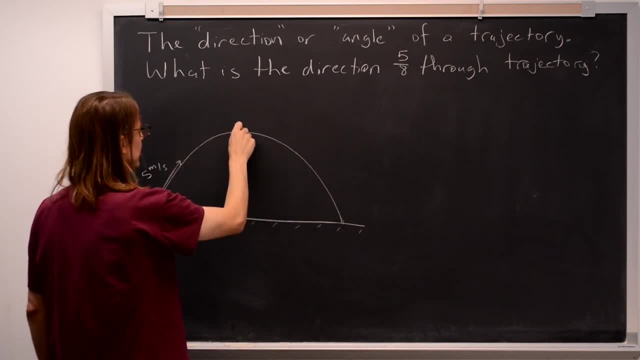 more interesting. I mean, you know, halfway through. these are even and symmetric, so this must be halfway through, so 5 eighths must be around here somewhere. So the question is, what direction is it traveling when it's right there? Because, as we mentioned in class, the direction of a trajectory. 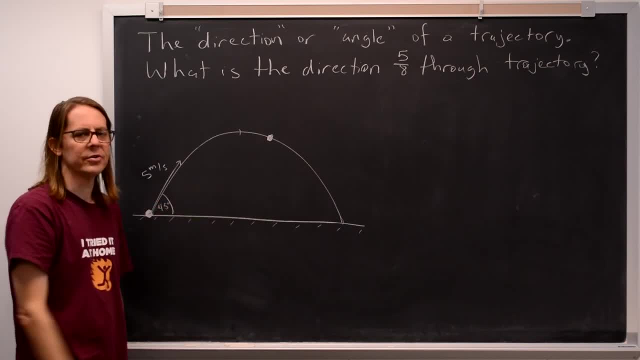 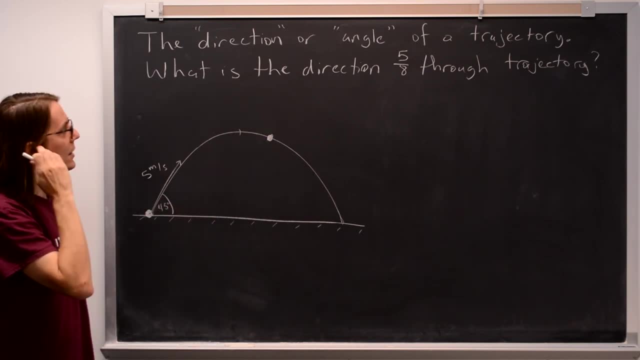 is based on the velocity vector, not the position of the acceleration. Okay, so the first thing we need to know is when this happens Exactly. So what we're going to do is: well, we need to know when it happens, because our general 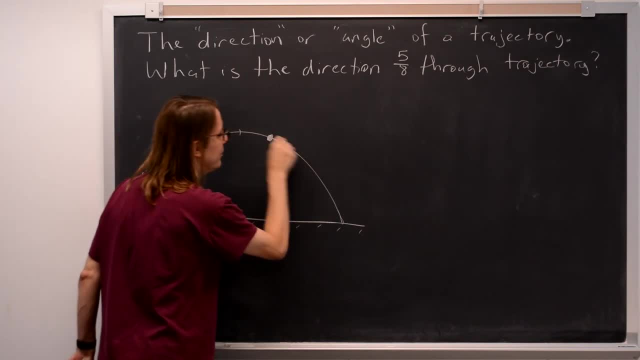 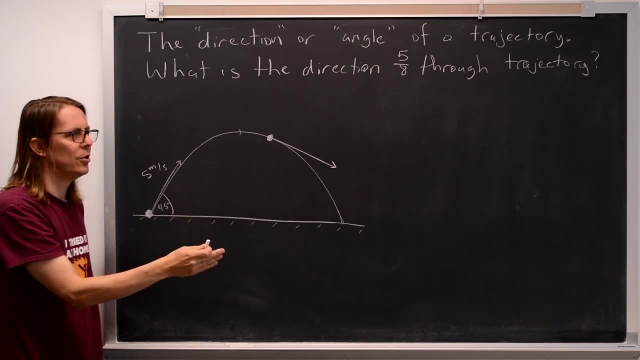 strategy. let me cover that first. our general strategy is to say there's a velocity vector at this point And to get the direction of that velocity vector we need its components. To get its components, we need to know when it happens. So the first step is to get the time. So what we're 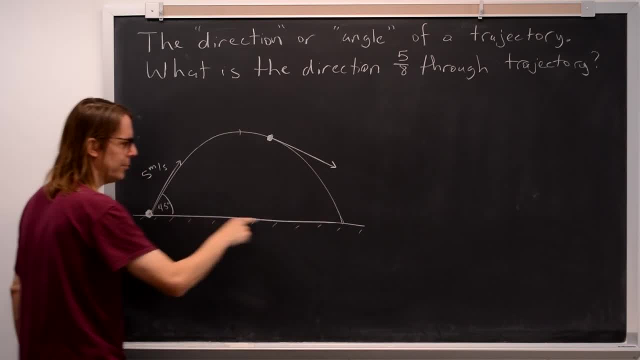 going to do is use our standard, even trajectory formulas to get the hang time, the time of the entire path, And then we'll just multiply it by 5 eighths. So you look up, you'll see that it's your T hang. I like to call it hang time because I'm such a sports nut- And it's 2 V naught sine. 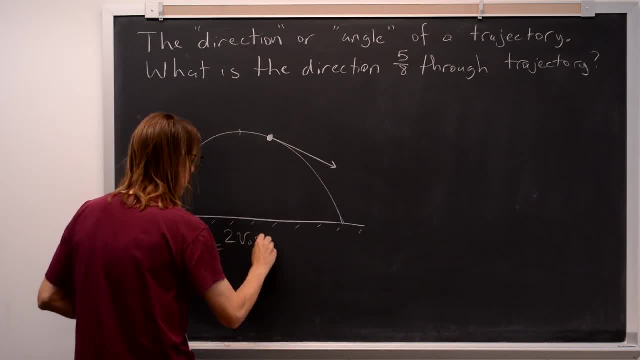 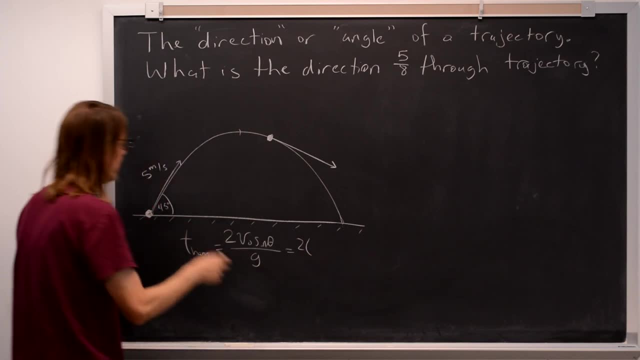 theta over G. We derived it in class. It's okay just to use the formula in this case. There you go, So we plug in 2 V. naught means the speed. the 5 meters per second squared Sine of the angle is 45. 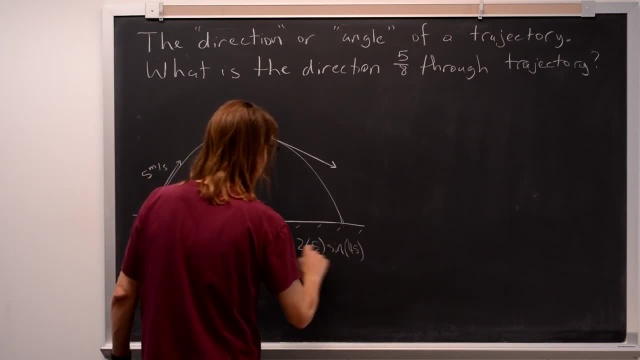 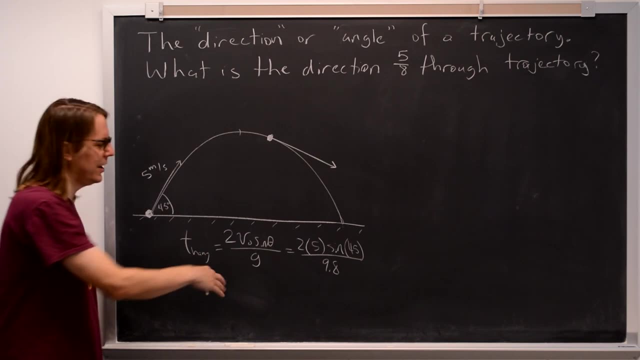 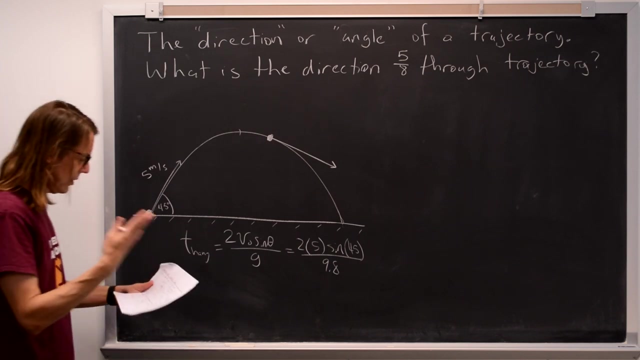 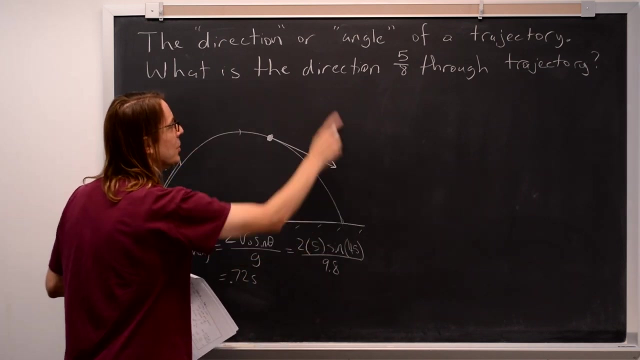 degrees And then over 9.8.. And we're using a negative number because this is a formula for a time we've derived. The negative was taken care of before. Just put the magnitude of the gravitational acceleration there And you will get 0.72 seconds. So that's the time to go all the way across. We want 5 eighths of the time. 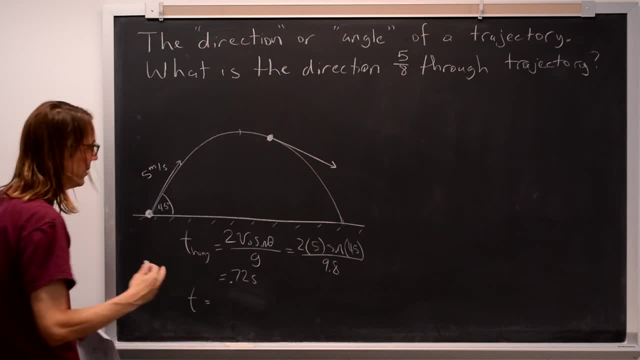 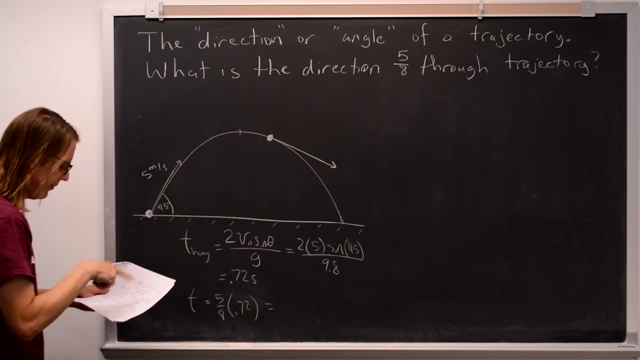 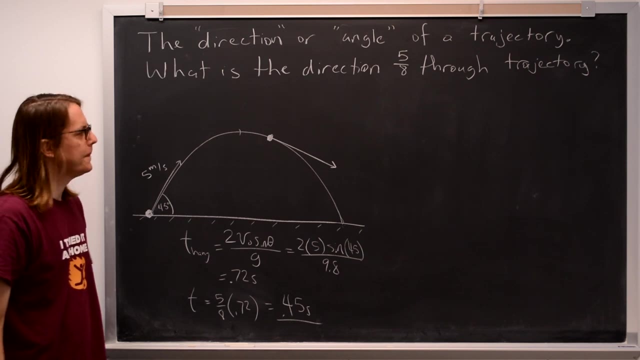 So I'm going to say T now. T is the time we're interested in. The time that that happens is 5 eighths times 0.72 seconds, which is 0.45 seconds. So that's when this happens. Okay, So now we just got to think about how the kinematics evolve and 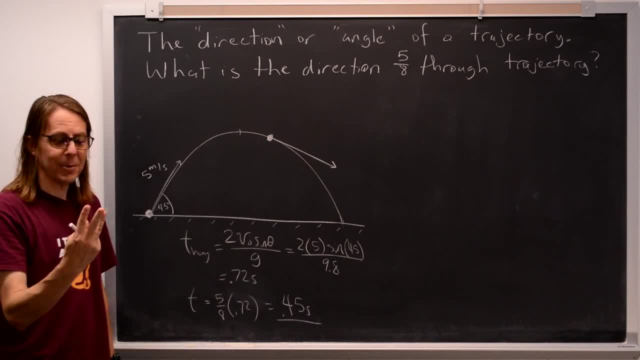 what's happening at 0.45 seconds, And there are three kinematics equations that you ever use. There's how the position evolves in time, There's how the velocity evolves in time And then there's where you combine them to get the what happens when you have acceleration for a distance. So 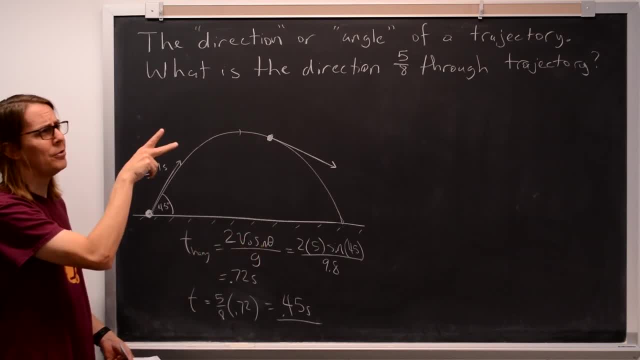 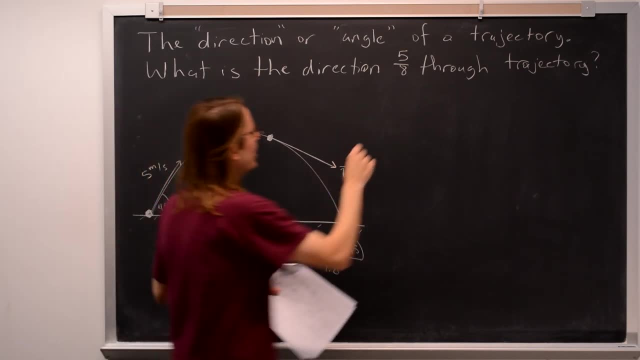 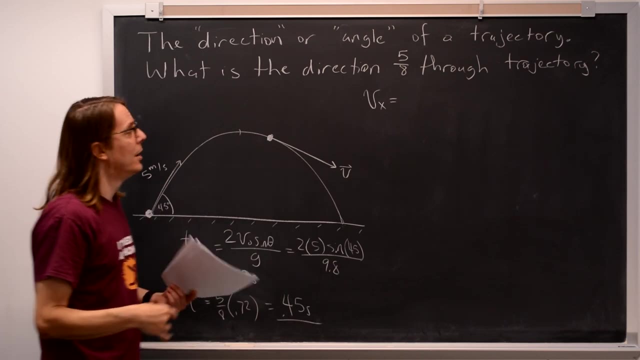 here we have the time 0.45 seconds, So it's one of those first two, But we care about velocity components, So it's that second what I said We want to think about: how does the x component of the velocity evolve over time? Well, Vx is Vx naught, plus acceleration of 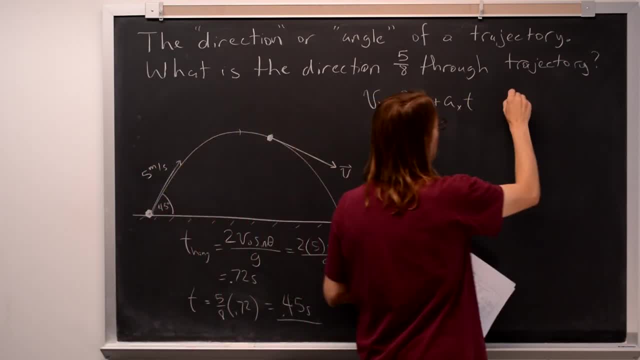 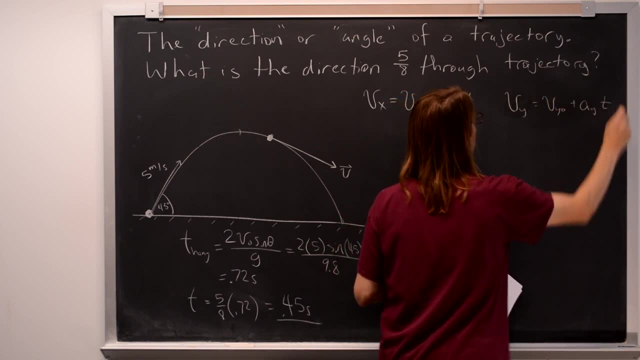 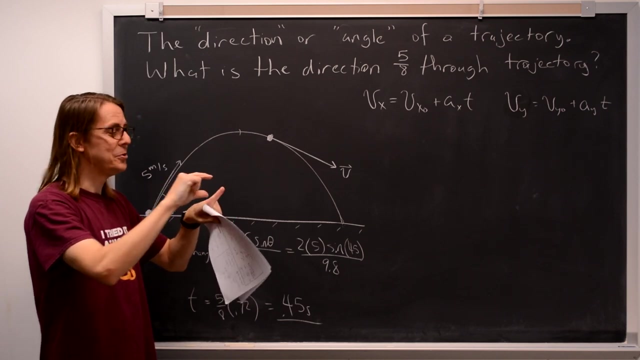 the x times time And for y Vy is Vy naught plus acceleration of the y times time. You don't even have to memorize this separately. Really, if you took your position, evolution equation: y equals y naught plus Vy naught t plus 1 of Ay t squared, you could just take a derivative. 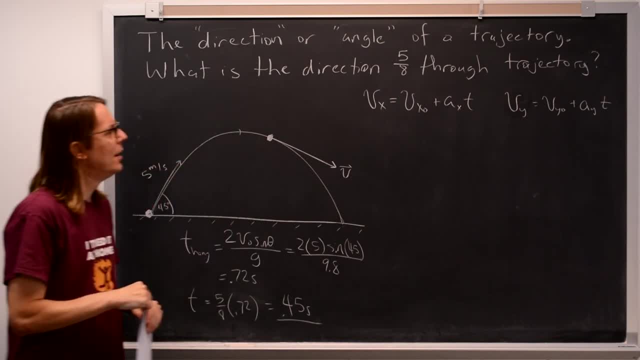 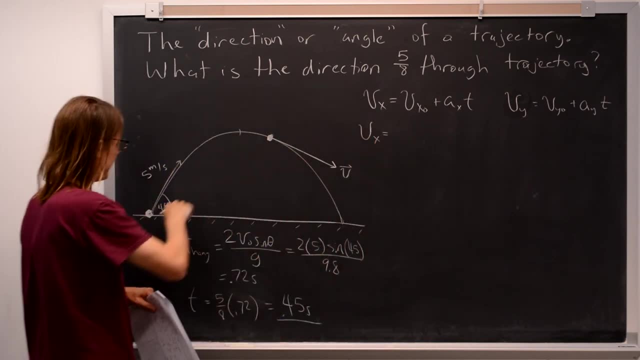 and get to this. It's really just calculus. Anyway, let's look at this and see if we get these two components. So Vx naught is the initial right. So it's 5 times the sine of 45,, 5 meters per second. 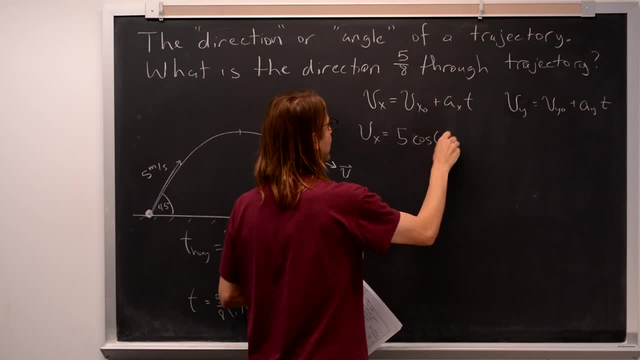 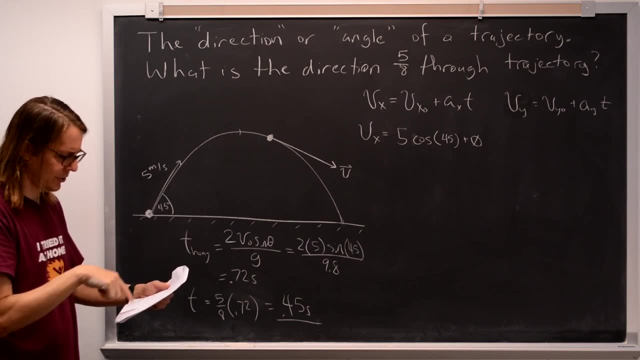 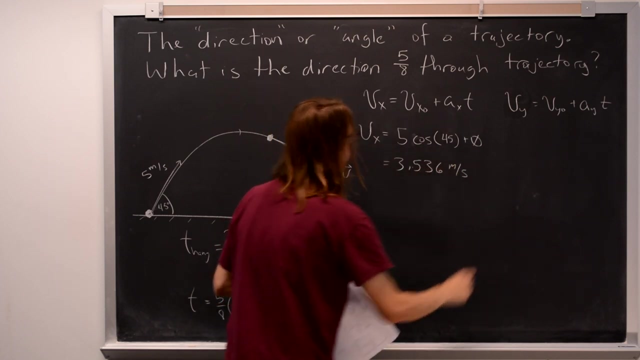 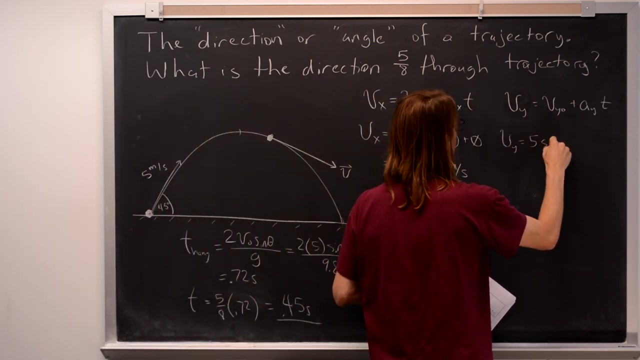 Oh, x is the cosine, 45 is the same Plus 0. It's not accelerating the x, It's just moving in the x. So the x component comes out to be 3.536 meters per second. Y is slightly more complicated. Vy is just 5 times the. 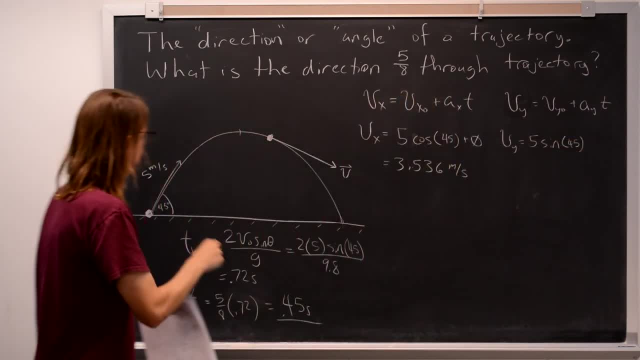 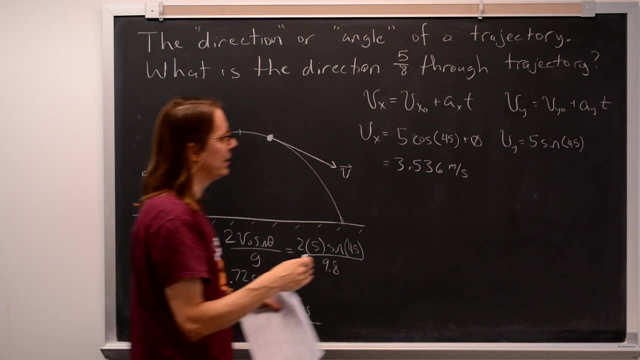 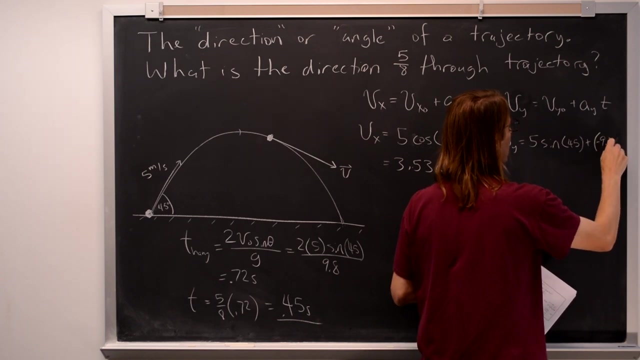 sine of 45. That's to get the vertical component of the motion And it is going to evolve in time because it is accelerating. The y is accelerating at negative 9.8.. And for how long? 0.45 seconds. 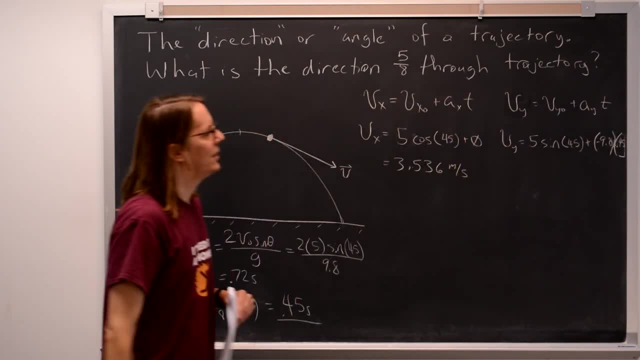 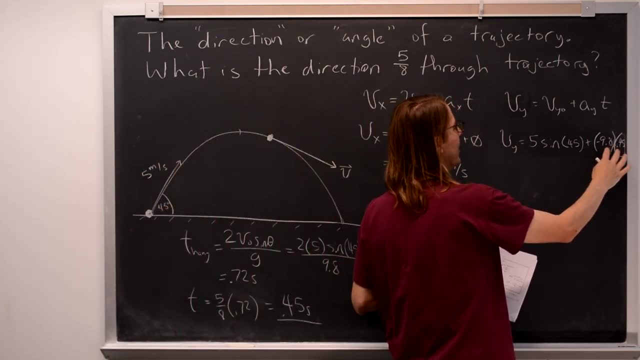 Sorry about that. That's 9.8 times 0.45.. So minus 9.8 times 0.45.. It turns out this value, this negative value, is bigger than this positive value, So it leaves you with a negative y. 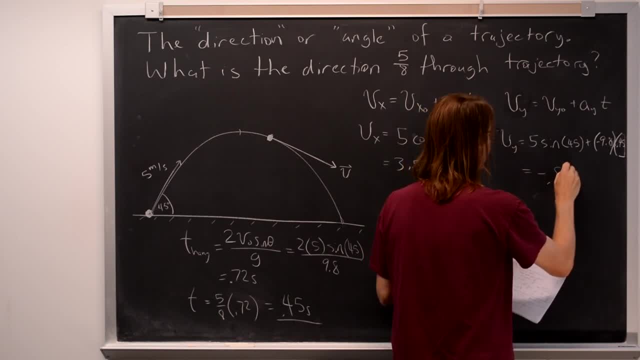 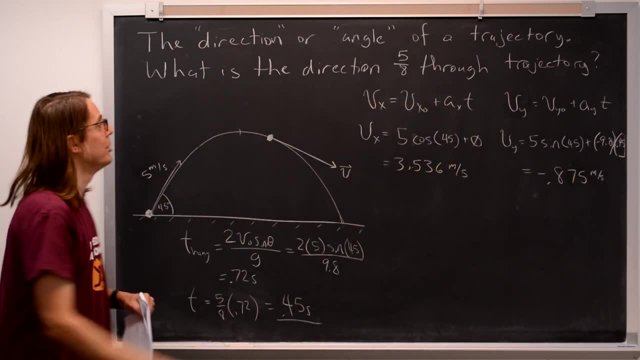 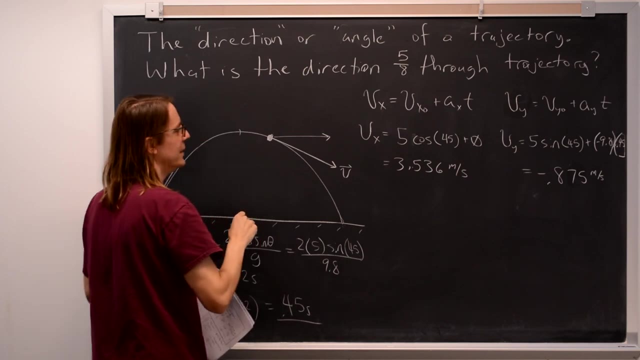 component of the velocity, A negative 0.875.. And that is what you would expect, because it is past the halfway point of the trajectory. So the x component just remains constant- That's what it was in the beginning- And the y component you would expect to be negative. The number is negative, Sure. 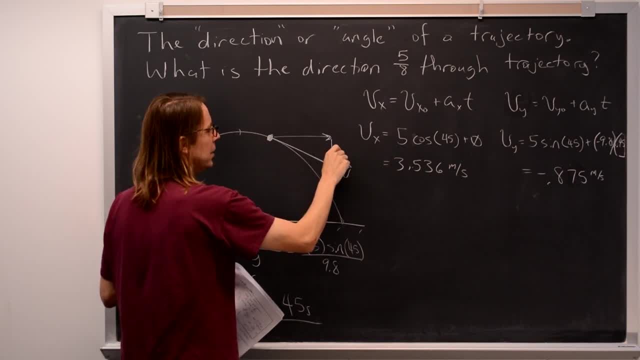 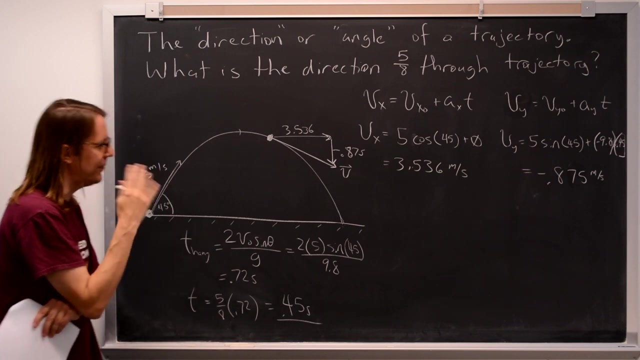 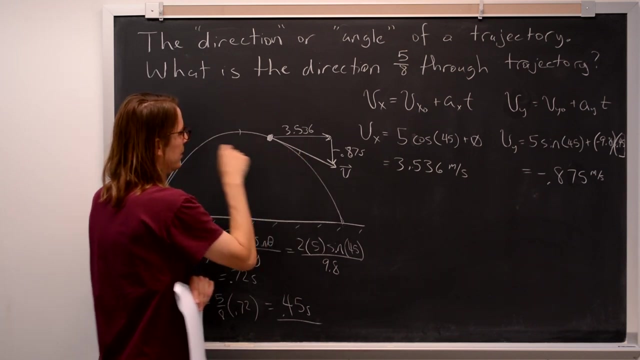 enough, Let's go ahead and draw it right here. So this was 3.536.. And this is negative 0.875.. I drew it that way to help you see the angle If you are not infinitely familiar with what trigonometric function to use. next, let's say the angle here looks like that, Or the 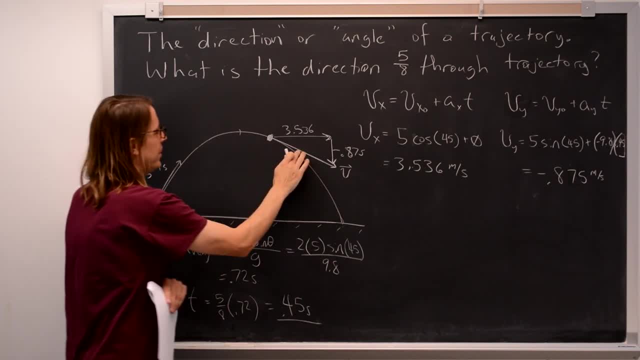 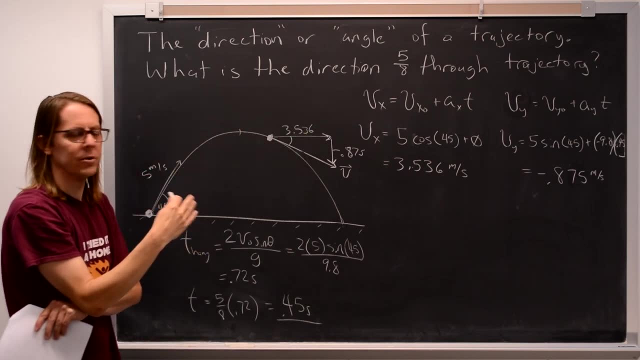 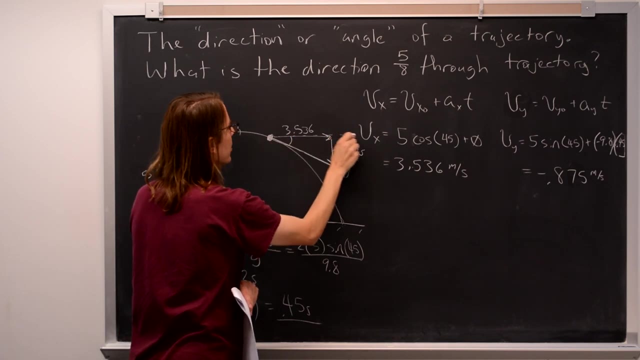 angle to the trajectory. Or, I'm sorry, the angle to the trajectory is here. What angle is it relative to the x-axis? Remember, the standard definition of a polar angle is: what is it relative to the horizontal? So the velocity vector we care about is here. Here is the horizontal. So there's the angle. 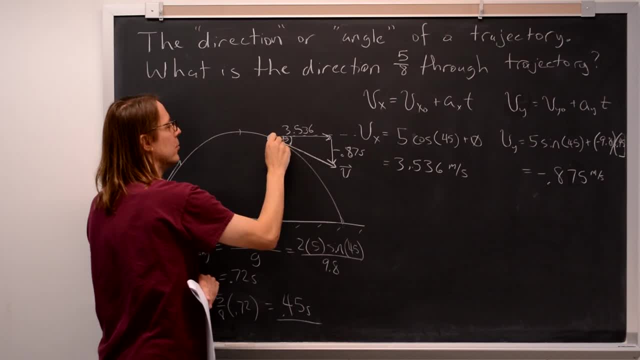 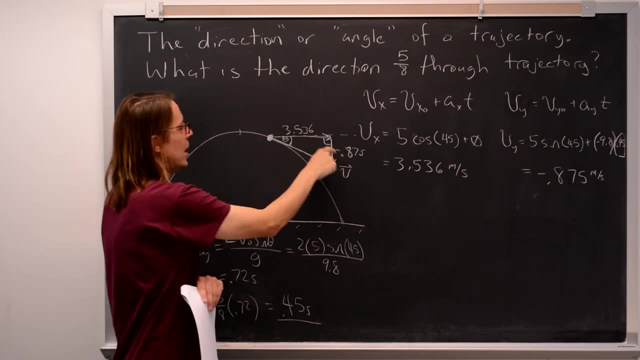 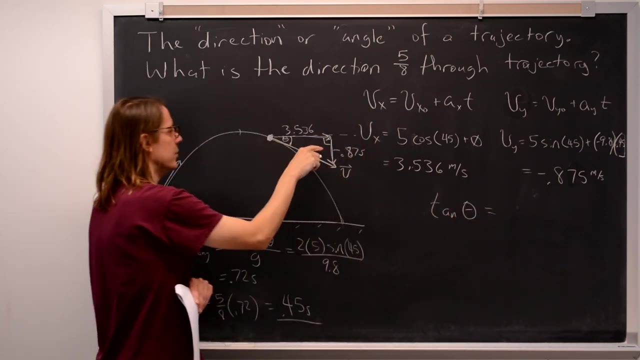 we want- And I went ahead and drew vy over here- to make a right triangle. So you can see, there's the right triangle. So we have the opposite and the adjacent sides of the triangle, So we're going to use tangent. Tangent of that angle is TOA, opposite over adjacent. 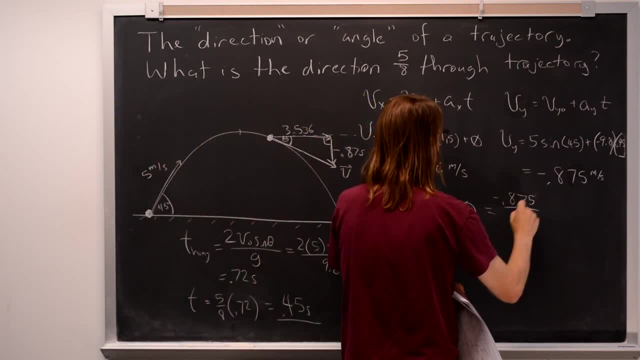 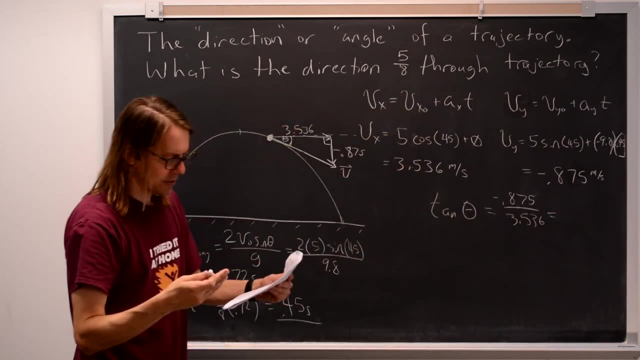 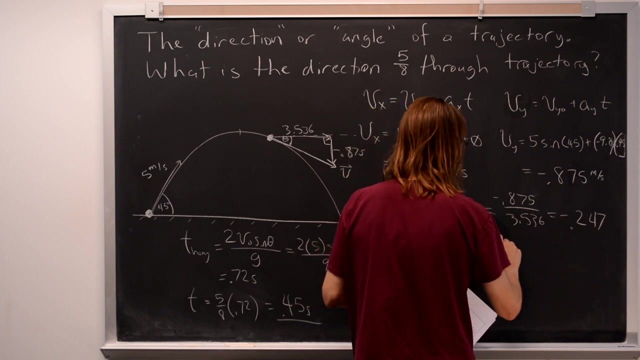 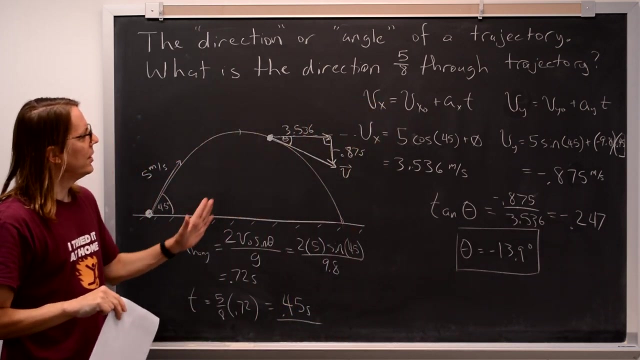 So negative 0.875 over 3.536.. And that comes out to negative 0.247.. About: it depends on how you round And you take the inverse tangent and you get about negative 13.9 degrees. So we look at that and we say, is that about right? Yeah, that's about right Once you're. 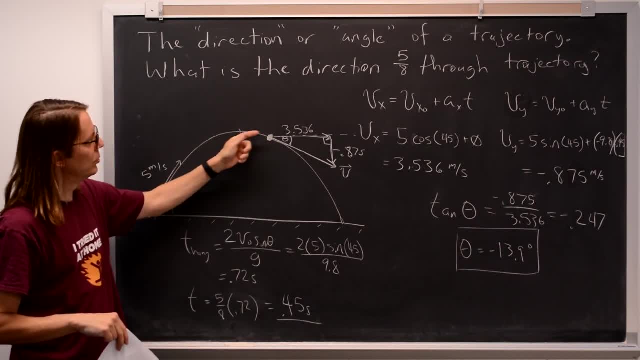 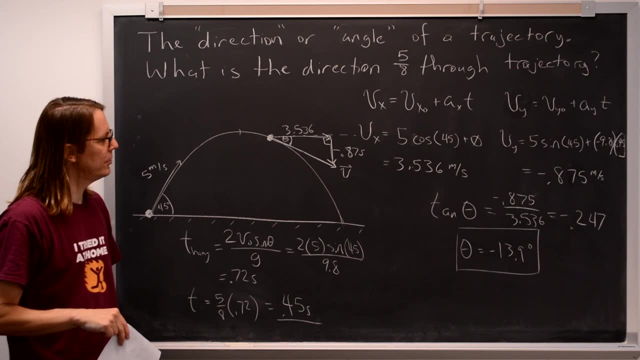 a little bit past halfway you're going to have a small negative angle that will just grow as you go down. So negative 13.9 seems reasonable, Okay When you're just a little bit past halfway through the trajectory. Had we solved it for this point, we should have gotten zero, Because at this point the